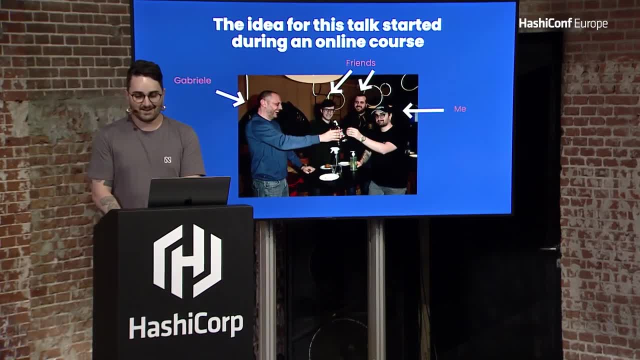 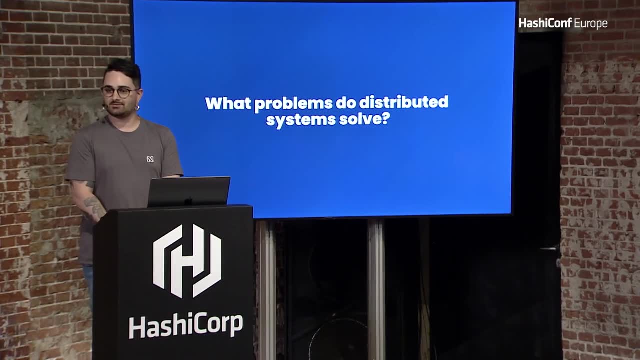 So this is me with my friends and Gabriele, And the problem was what problems do distributed systems solve? right? It's not easy to make junior developers understand that concept, especially for, you know, non-technical people to get into distributed systems. So we're. 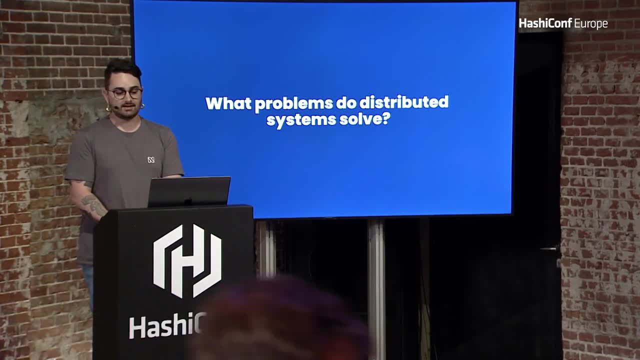 not sure if this is a good idea to do, but we wanted to give them an idea of what distributed systems are. We wanted to do something to let them understand this, and so we came up with the idea of talking like to a five-year-old guy and see if we can try and teach something. 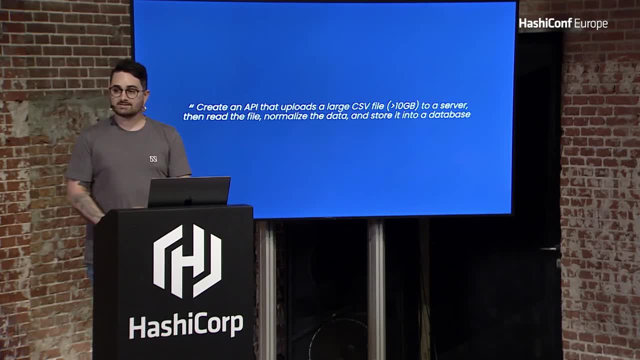 But we started with a very simple requirement. So we asked them to create an API that uploads a very large CSV file, which must be greater than 10 gigabytes in size, to a server. Then, once we have the file, read it, normalize the data and store it in a server And we 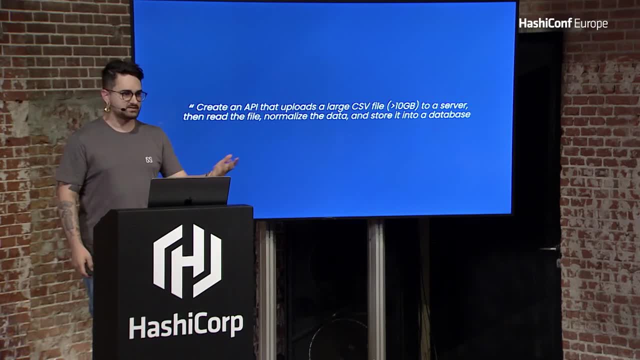 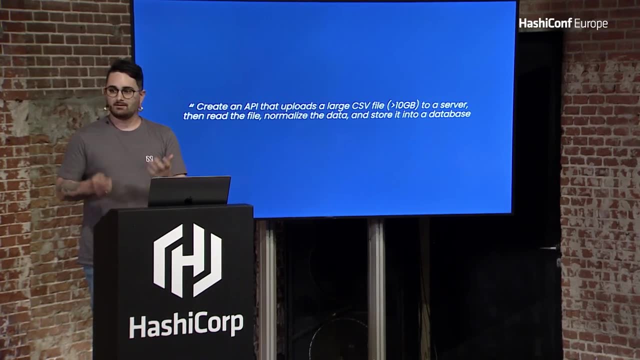 into a database. That's not just nice as an exercise, but also as an interview question, in case you're looking for good interview questions. So the vast majority of the students came out with the following diagram: right, So we basically are users. 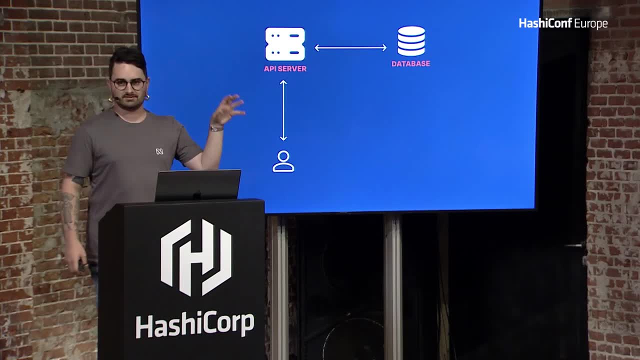 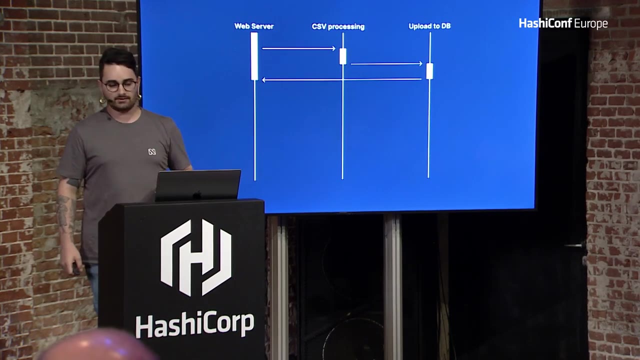 We upload something to the API server, The API server takes the CSV files, normalize it and uploads to the database. So if we go in a diagram, in that kind of diagram, we will see that we make a request, Web server process, the file uploads the data. 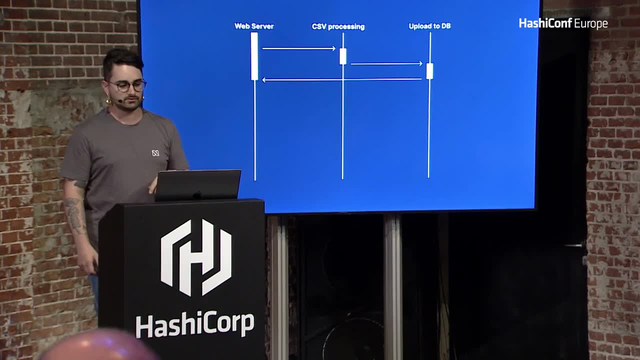 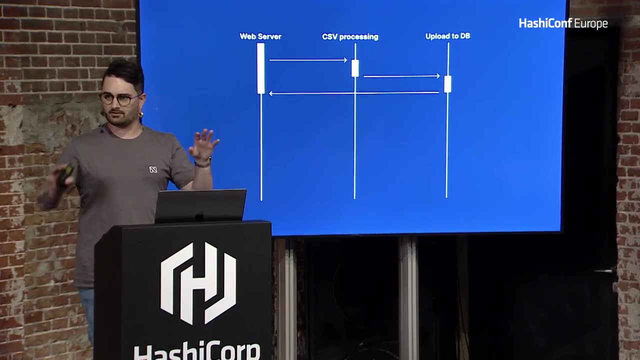 into the database and after that sends a reply to the final user, And that could take, like I don't know, 30 minutes. It depends on the internet connection you have. I'm from Italy. Internet connection here is really, really bad. 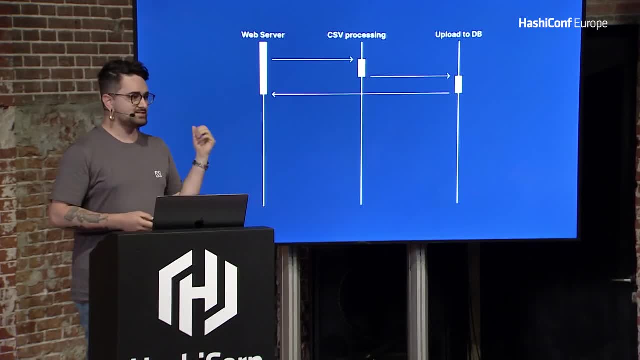 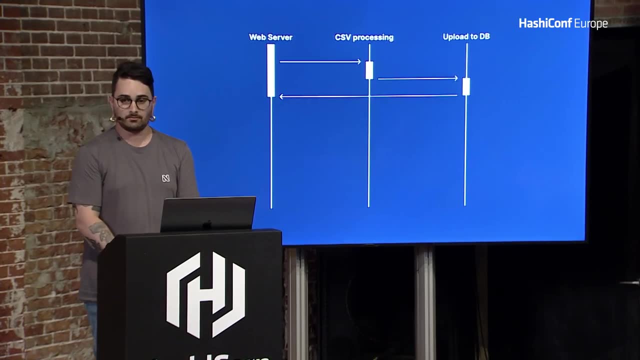 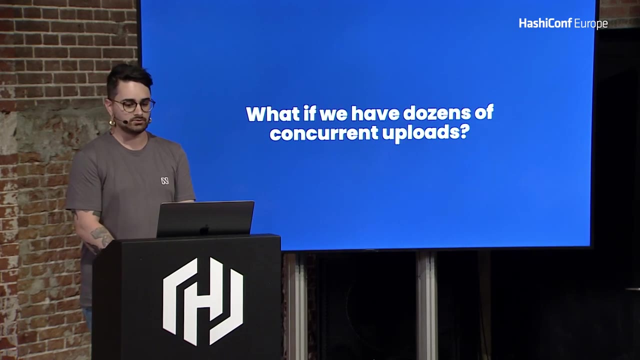 so you don't want to go that way. Also, this is a synchronous operation, So that means you are blocking people from uploading multiple stuff concurrently And, in fact, the biggest problem we pointed out during the review for this architecture was what happens if we have dozens of concurrent uploads. 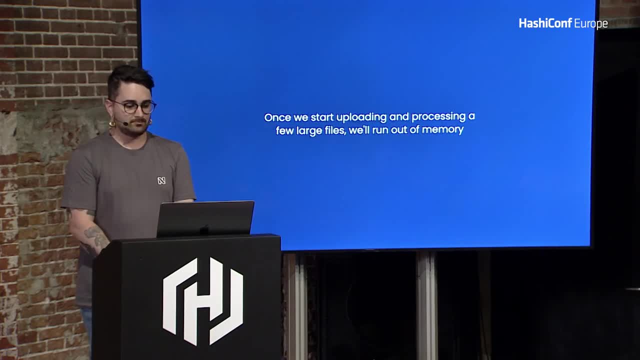 So it was pretty easy. We start uploading and processing a few large files and we run out of memory. So after that the most advanced junior developers in the course said: OK, great, So why don't we just take a load balancer? 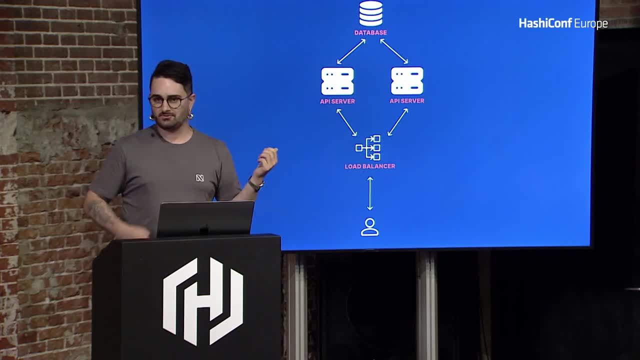 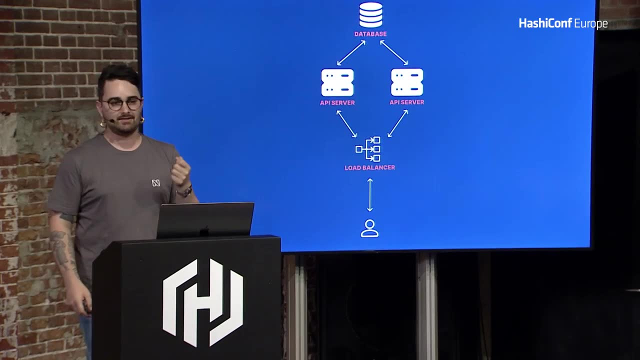 We create a couple of servers and if one is busy, we can write direct to the other one and we can scale horizontally like forever. True, it's part of the solution, but doesn't fix the problem. So this is what I want to introduce you: the ice cream. 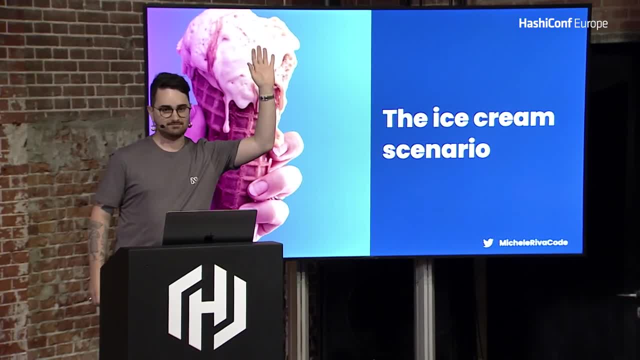 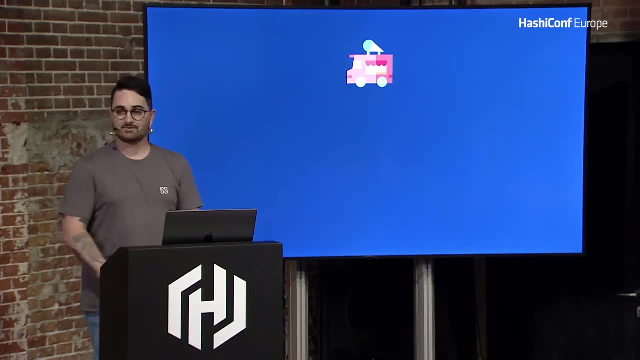 scenario. So who loves ice cream? Awesome, OK, cool, You're going to like this. So let's pretend you're an ice cream maker and you have a beautiful ice cream truck And eventually you're in Amsterdam and you find a lot of people, which is really angry. 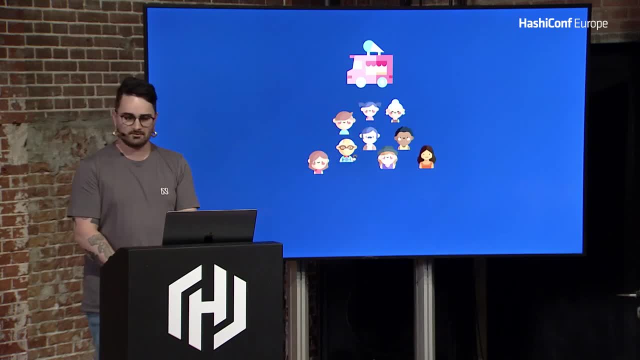 and they all want ice cream. So there is a lot of people And as people came by, you start distributing ice creams, but you don't have enough capacity. So there is a lot of people and people continue to increase and there's nothing else you can do. 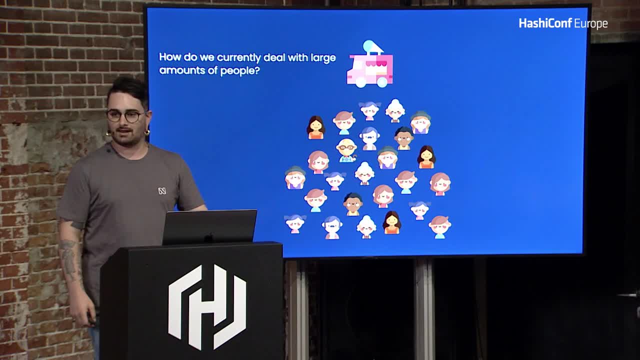 So how do we deal with that kind of problem in real life? Any suggestion: More ice cream trucks? That's true, But before getting new ice cream trucks we have to deal with the problem. So we create queues, Then we get there. 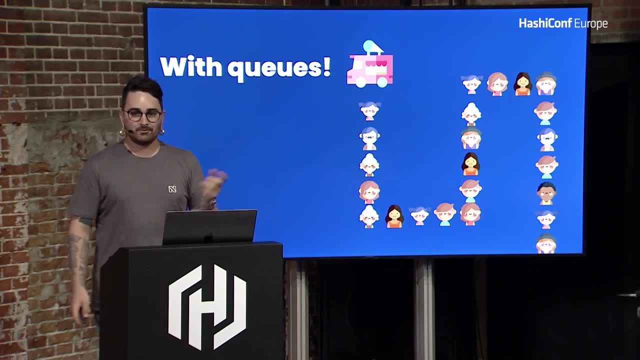 You're totally right. So, yeah, we can start creating queues, But what happens if we really have a lot of people? You know there are kids and people treat kids poorly or so tries to cut the line, whatever happens. So we want to ensure that the first person arriving 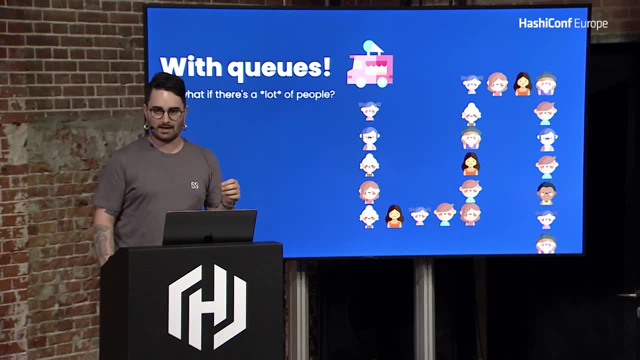 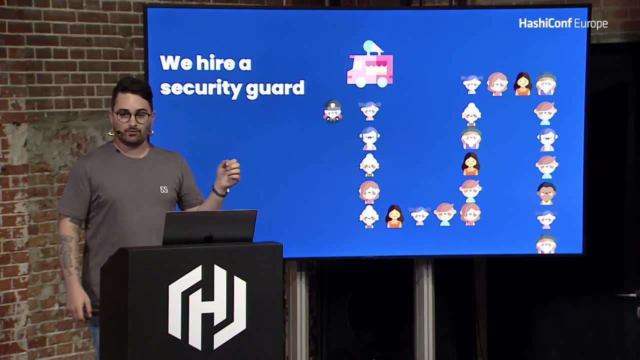 to the ice cream truck will be the first person to get served, right? So we hire a security guard And that boy- sorry, that girl- will make it sure that everyone will get served in the correct way. So if I'm the first, I will be served first. 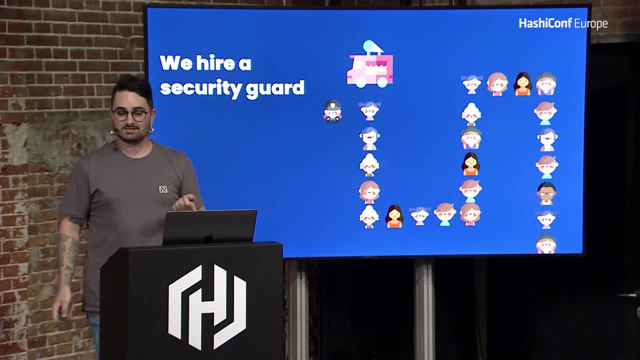 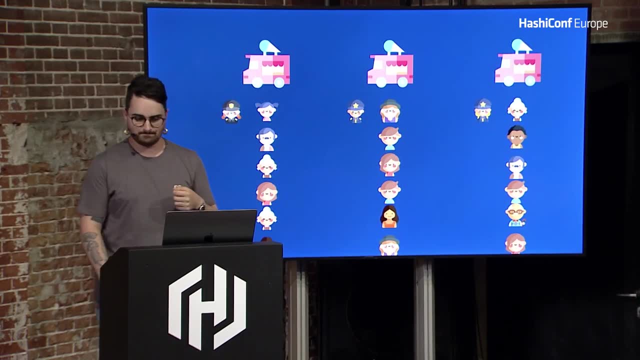 And, of course, like we were saying at a certain point, a single queue is not enough. So we'll get more ice cream trucks, more guards And we can scale in many different ways from now, But of course, when it comes to software architectures, 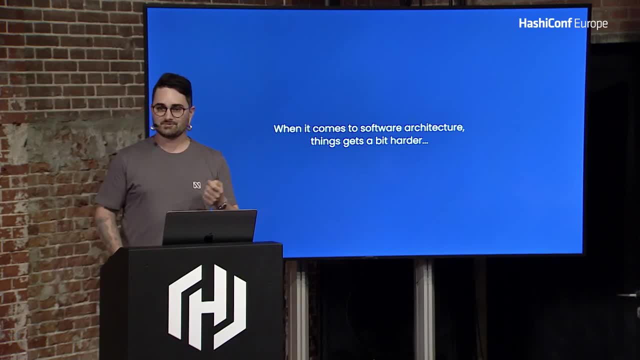 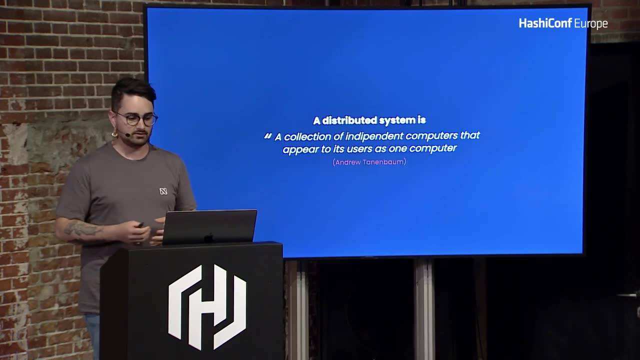 things get a bit harder, right. So this is where we want to introduce the concept of distributed systems. So a distributed system? A distributed system, by its definition, is a collection of independent computers that appears to its users as one computer. That means that it doesn't really. 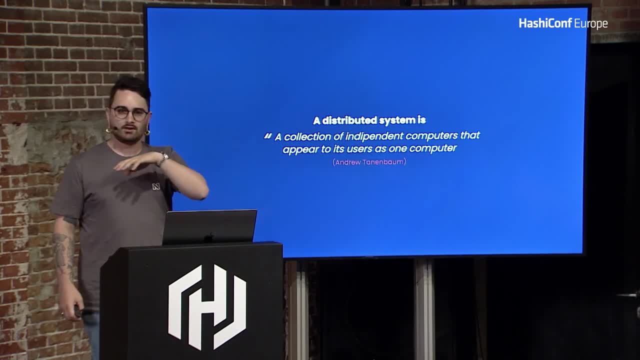 matter if we have like 10 ice cream trucks, if we have 100 ice cream trucks or one single ice cream truck To the final user. what matters is the speed and the possibility to ask for many different ice cream at the same time. 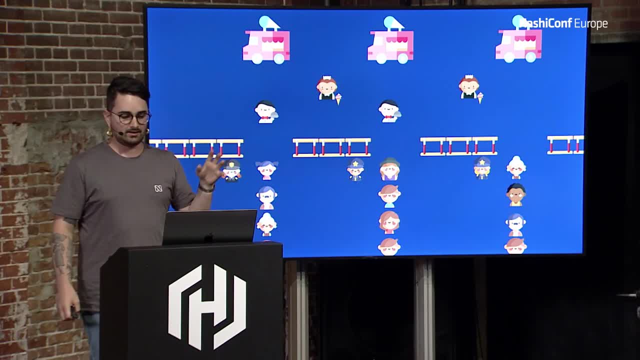 So we end up in a similar situation. We don't really care If we see ice creams, we only wait for waiters and waitress to give us our ice cream. right And to call a system as distributed, it needs to respect three distinct rules. 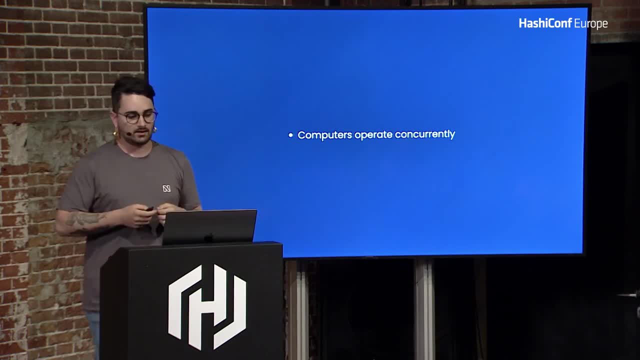 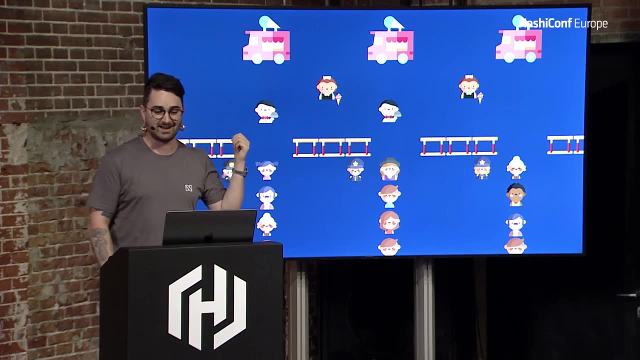 First of all, the computers in distributed systems needs to operate concurrently, And that's the case. So it means that if we are in the first ice cream truck, it operates independently from the other trucks, And also for the queue and for the waiters and waitresses. 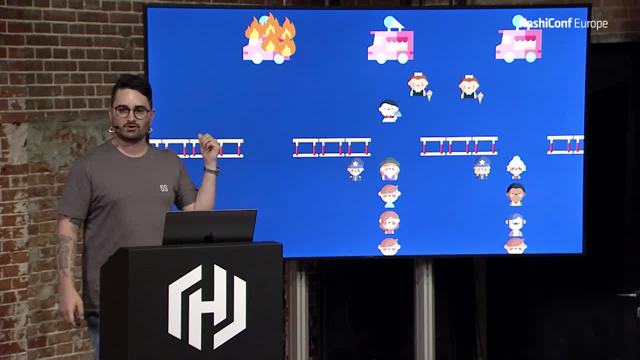 All computers fail independently, which means that if an ice cream truck is on fire, it doesn't affect all the other ice cream trucks and definitely don't want to affect the waiters and the waitresses. And here we come to the most complex topic. 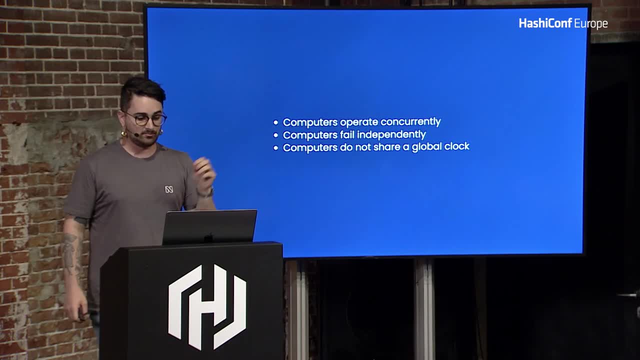 when it comes to distributed systems. in my opinion, of course, Computers do not share a global clock. What does it do? It doesn't share a clock. It doesn't share a clock. What does that mean? Let's say we have a couple of watches. 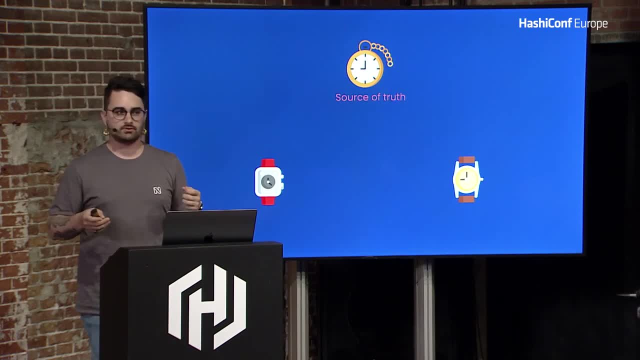 And we want to synchronize them to a unique source of truth. So we know for sure that the golden watch in my slide is the correct one, pointing to the correct hour, And we want to synchronize two different watches to that hour. Well, this is technically speaking. 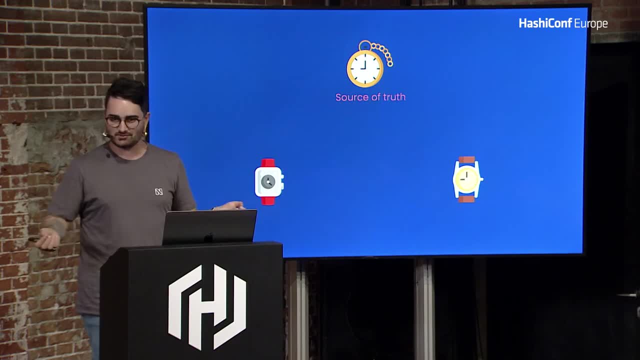 impossible due to the current laws of physics limitations we face every day, And that's because when I make a synchronizing request, I make that request in a certain period of time And there is some latency to reach the source of truth, And also there is some latency in the response. 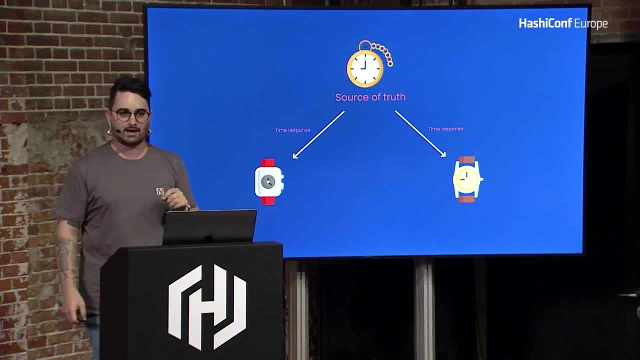 So we can get really, really close to a correct hour, But we will never have synchronized hours And if you think of that, for example, if I look at my watch right now, we have a limitation, which is the speed of light. 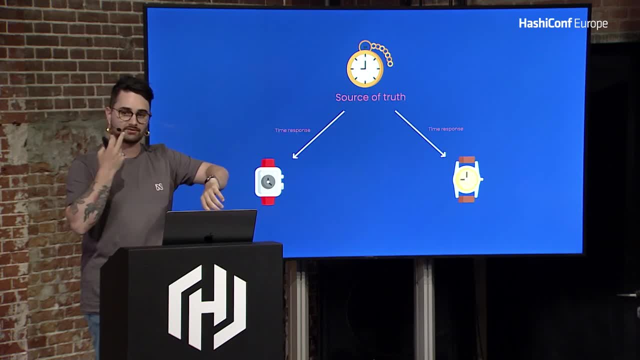 So the light needs to be reflected on my watch and go back to my eyes, And this is latency, which is really tiny in that case, still exists. So we don't want our system to depend on clocks because they are not reliable in that sense. 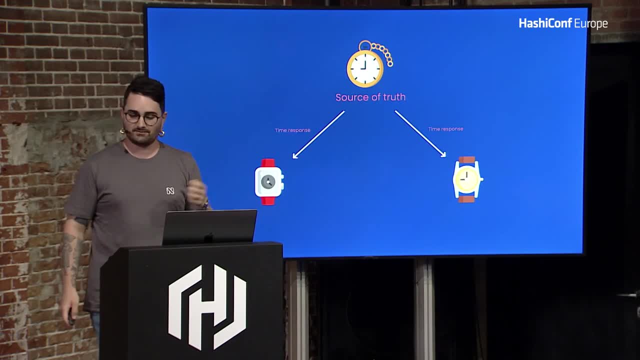 Of course, there are a couple of standards for dealing with that kind of problems, And I just can quote them, like Network Time Protocol NTP, and Precision Time Protocol- PTP. There is an awesome article on geeksforgeeksorg. 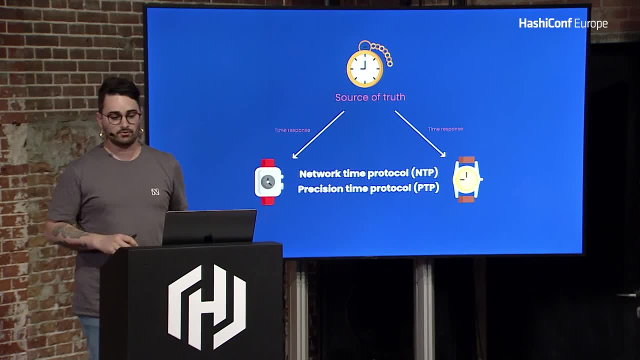 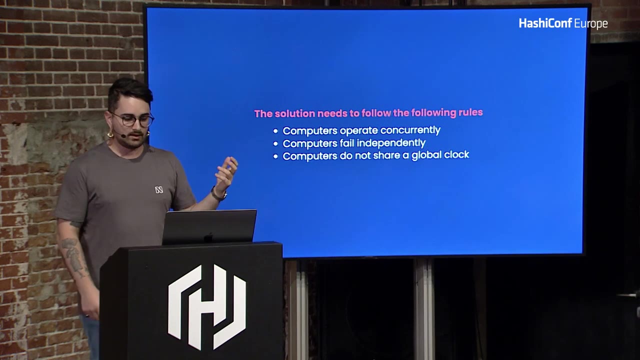 that explains those topics in depth. So I highly recommend you looking into those if you are interested in that topic. So from now on, the solution we require to the students was a solution that could satisfy the following requirements. So the system, all the computers in a system. 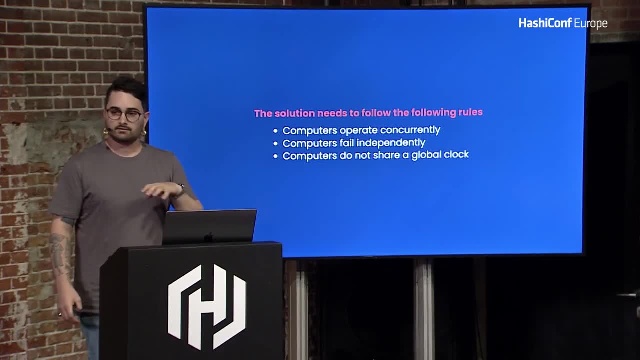 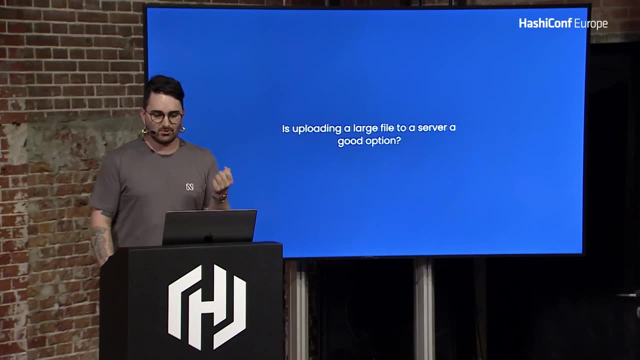 had to operate concurrently, independently, and they doesn't have to share a global clock right. So let's start from the beginning. Was uploading a very large file to a server a good option in first place? I don't think so. That's true. It's because, for example, I work in Nodejs mainly and you don't want to upload files and serve files from Nodejs. Believe me, I love it, but that's not the best option, And that's also the case for other languages. 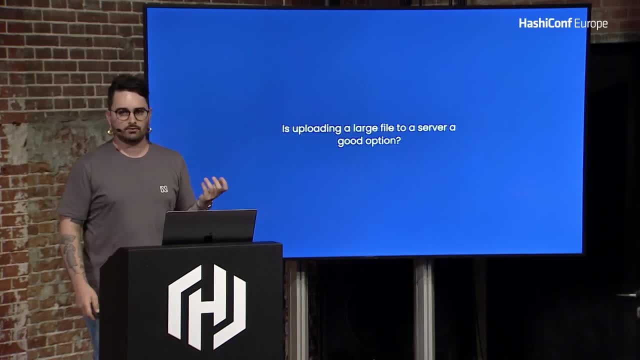 So I would go with a more structured way for dealing with large file inputs and outputs, And that's the case for object storage, for example. Doesn't matter if they are S3, Google Cloud Storage, Azure, Blob Storage. We don't really care about the implementation right now. 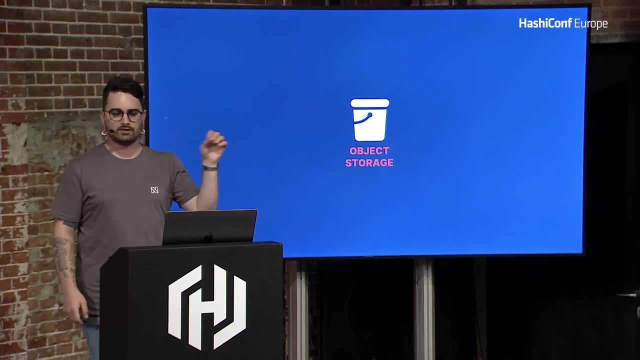 We just care about what we are doing. So after we upload a file to an object storage, we could trigger a change in what we call the waiter, for example in our ice cream truck, which in that case can be RabbitMQ but could also be a streaming service. 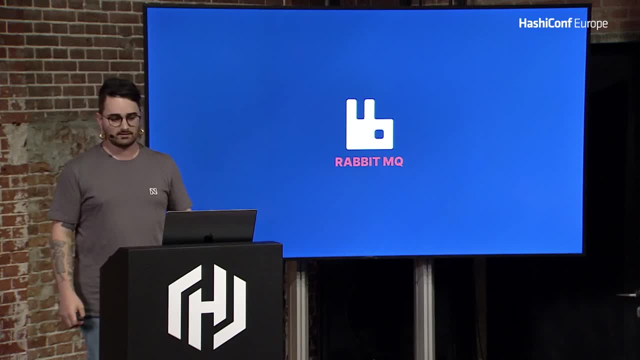 like Kafka. So we upload something to a bucket. Bucket notifies Rabbit And at this point, when a waiter is free, so they don't have to bring some ice cream to people in queue, they can go back And take a new ice cream. 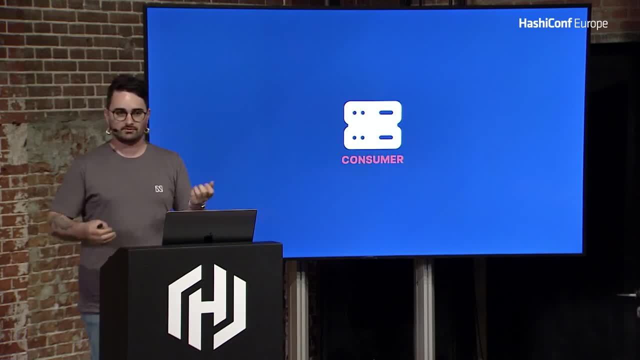 So we have the concept of consumer. So the consumer, when it's not doing anything important, will pull from the queue and will be able to process the file, And Rabbit will keep the queue in a first in, first out way, such that the first person reaching for the queue 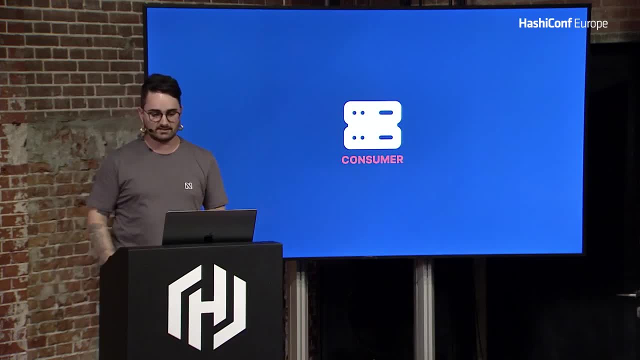 will be the first person to get served properly. So the consumer will send the data to a database And after we have the data in the database, we can eventually ask for this data from an API server so that we can query- for I don't know- e-commerce data. 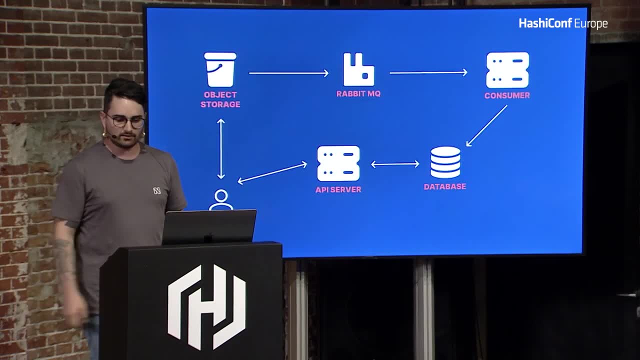 or whatever we need from that server specifically. So the final diagram looks something like that: We are users, We upload to an object storage our file And we can subscribe to an API server using WebSockets or whatever, so that we can get notified, maybe. 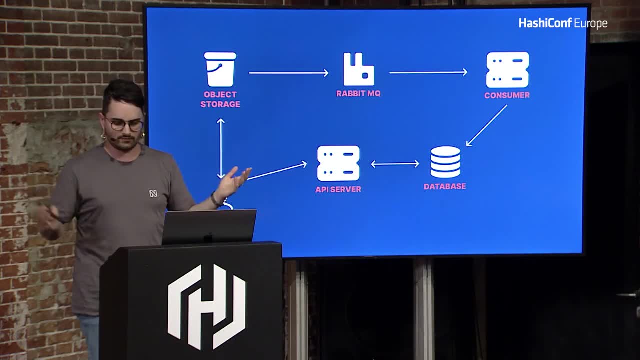 with a different queue on our message broker or Kafka or whatever. We can get notified when the process is done And we can start querying the database as soon as the data comes in. And also we fixed another problem. This is an asynchronous way of dealing. 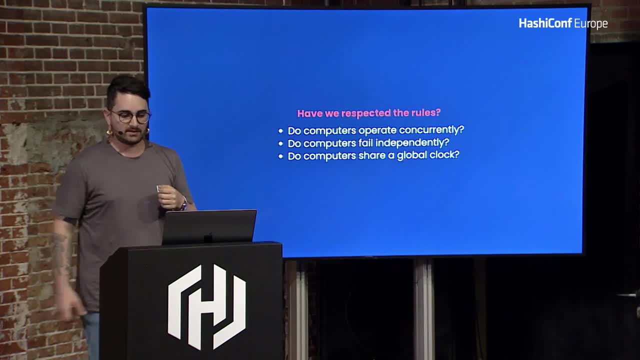 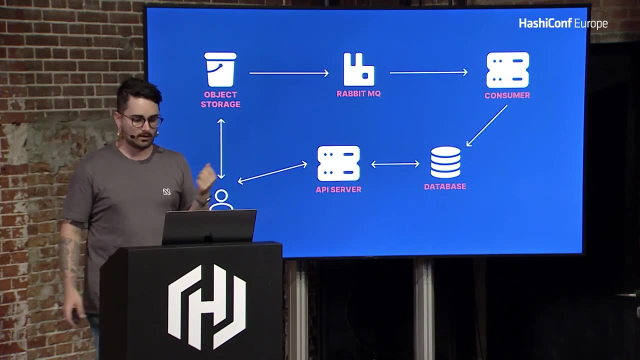 with that kind of problems. So have we respected the rules? Are the computer operating concurrently? I would say so. Do computers fail independently? Yes, they do fail independently. And you may be thinking right. OK, but if RapidMQ crashes at this time? 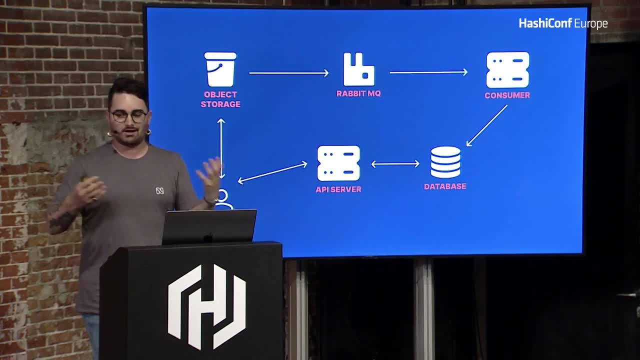 I'm not able to pull stuff. OK, this is totally correct. But you're likely to deploy them into clusters and whatever. So it's a very resilient software, So I wouldn't be super concerned about that. Do computers share a global clock? 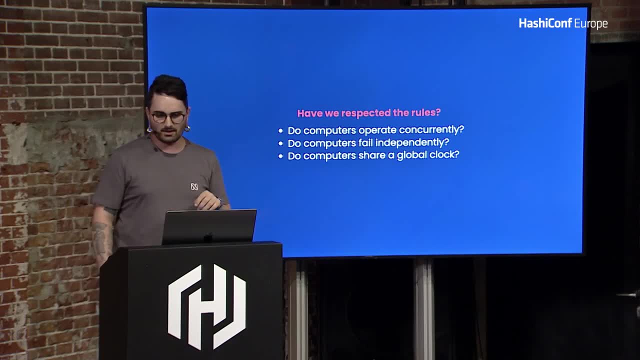 Well, we don't actually care about that, And that's because it's more something we need to care about when we are creating distributed software rather than architecture at this point. So what problems did we solve? Of course, we are not able to scale a very large scale. 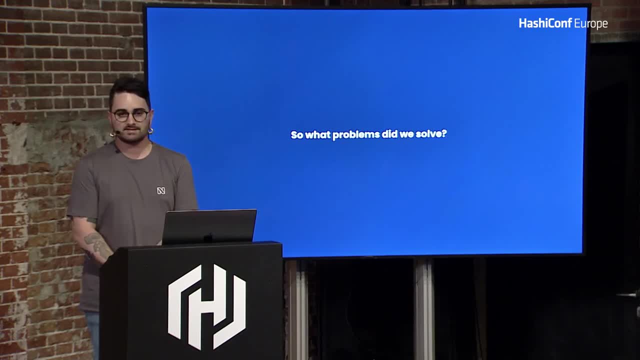 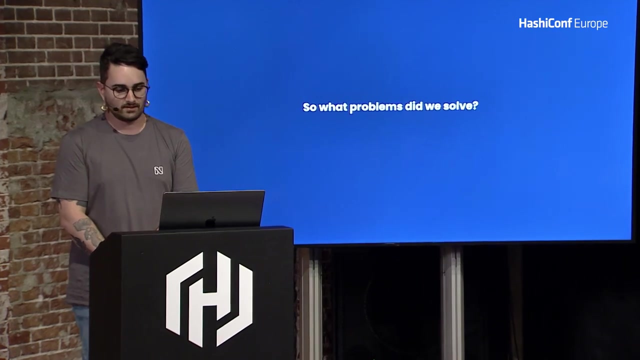 application very easily, starting from a very simple problem, And that's a lesson that I'd like my students to learn at this point, And maybe we can all learn something from simple, simple problems that can cause very complex solutions. So that was all for me. 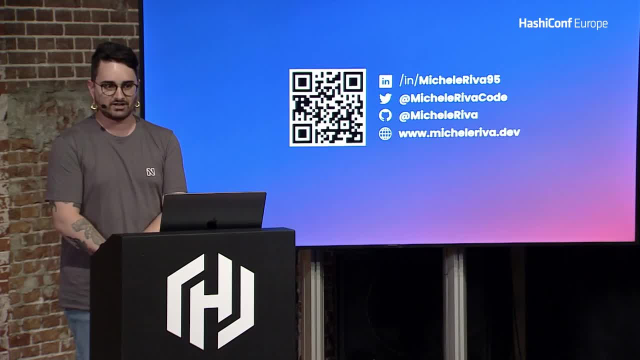 Thank you all for being here. I'll leave a couple of contacts just in case you want to reach out. And yeah, see you all around, Thank you.